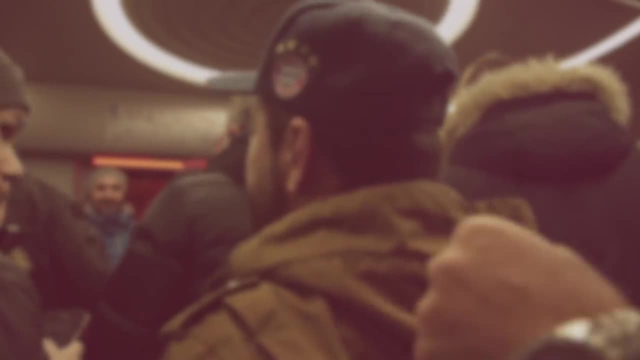 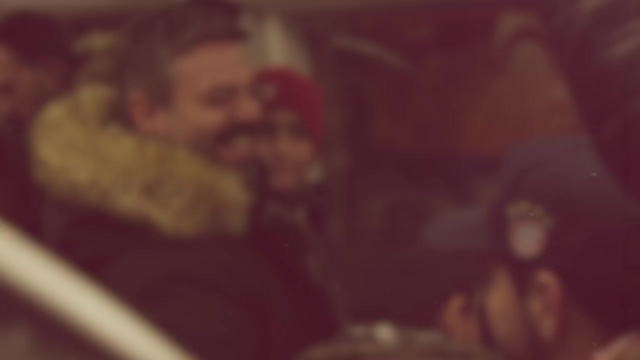 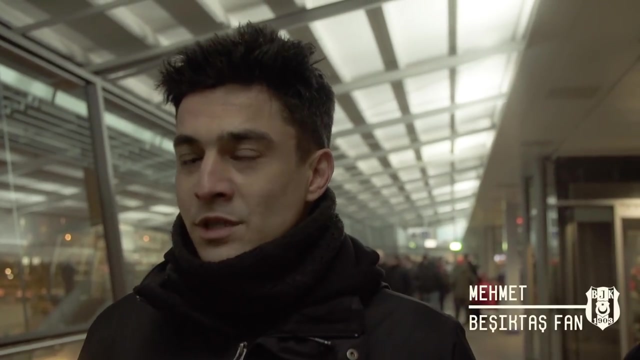 More safe? I doubt it. Our management decided not to send local supporters from Turkey to the Munich game because of the decision which had been done by UEFA after the Lyon-Besiktas game. We had some colleagues from Bayern Munich supporters, so they arranged us a dinner last night. 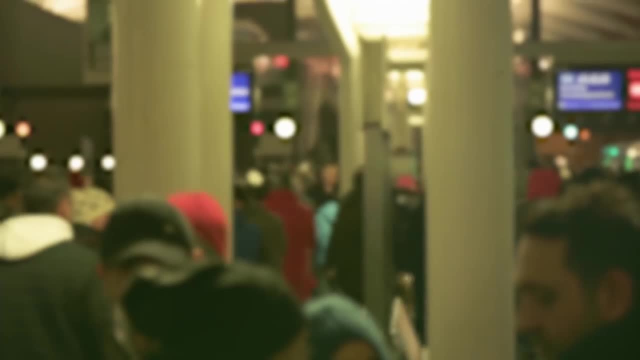 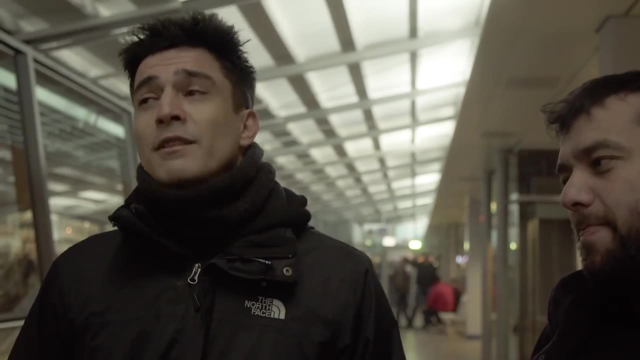 Today. they helped us to find tickets, because we can't find tickets that easily. As you may know, we have a huge immigrant population living in Germany. That's why most of the people, even though they are not supporting Besiktas, also want to join the game. 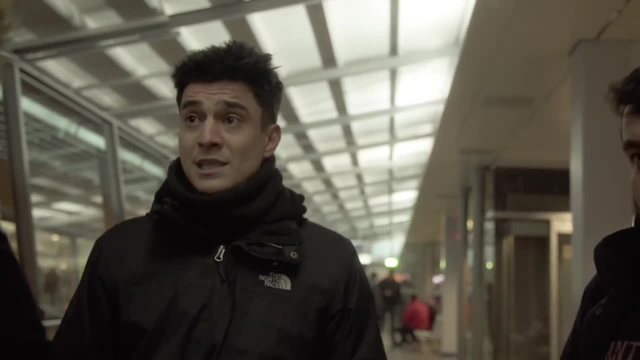 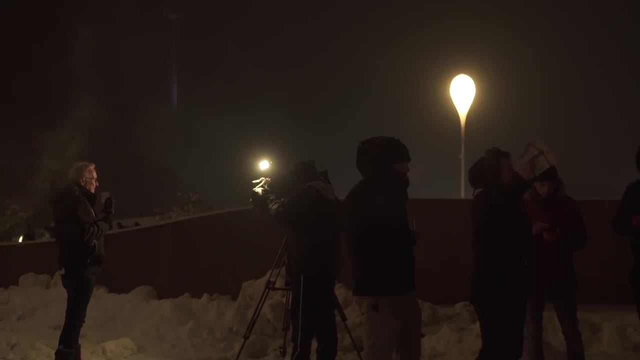 As far as I learned, they charge 100 euros, which is more than twice expensive than usual prices. The policy of Besiktas is not making any sense because they create a situation where the fans have to throw the law, don't respect the regulation, go in the home sector just because they want to support the club. 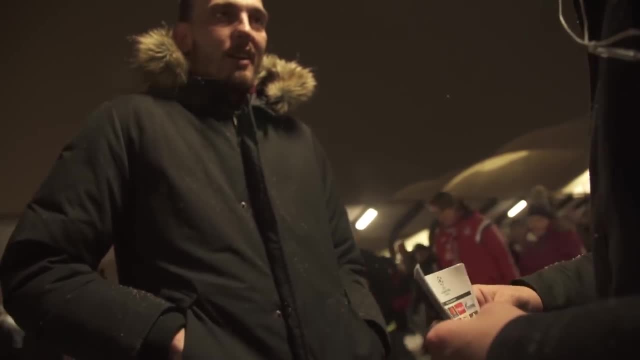 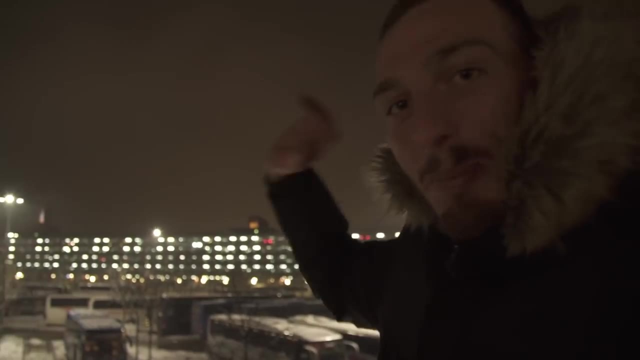 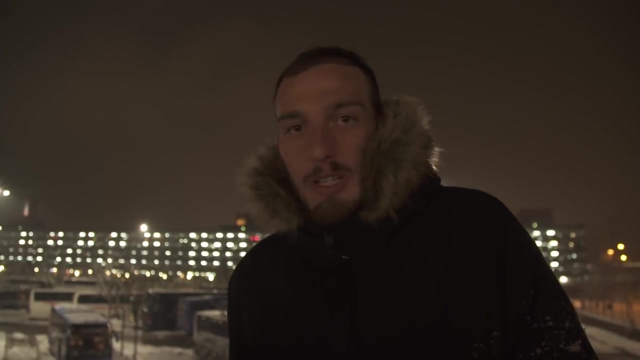 There are some Turkish guys travelling by these tickets, but they almost don't have jerseys on it. You come out here right now and you see a whole set of buses coming from all over the country. In 2018, when the club is a global product, who are you to say? what makes a Bayern Munich fan? What makes a Besiktas fan? 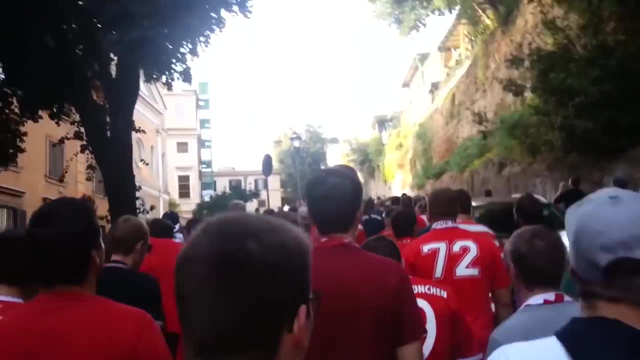 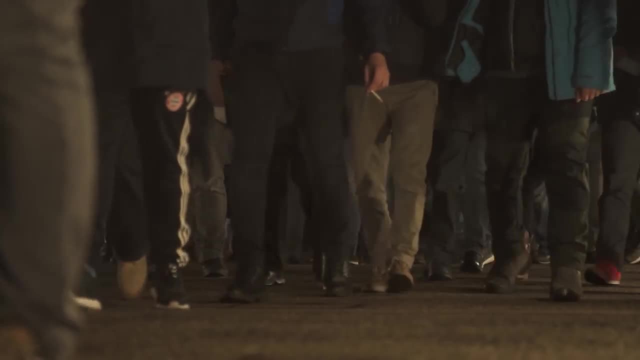 Those people who live all over the world, who follow these clubs, who try to attend their matches, And from far away, on television. it can look all beautiful and easy, But the truth is someone's going to get in trouble because one cop will see a ticket with somebody's name on it being sold to the wrong person and will be banned for life. Is that the supporters' fault or is that a legislation system that isn't taking into account the real practicalities of being a football fan? You find yourself in a situation where the club does not defend you, UEFA makes no rules and you have to rely on opposing supporters to go to a football match. 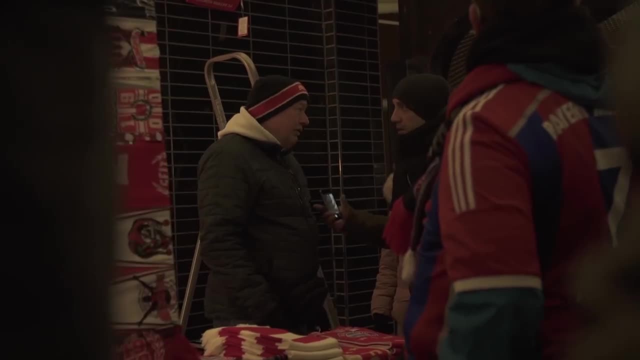 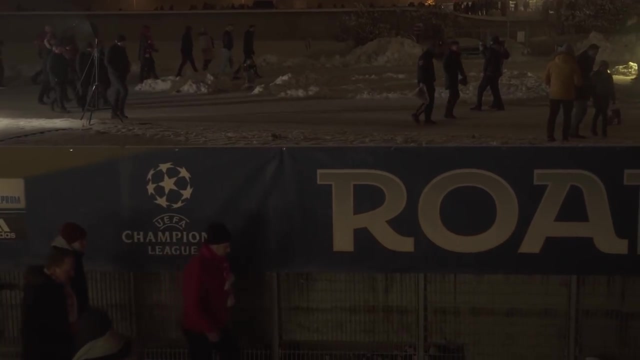 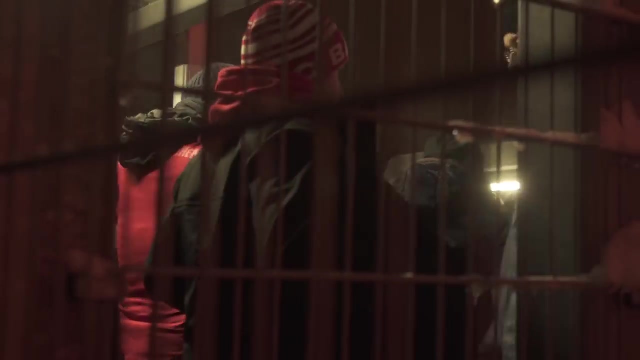 I believe just football fans always find a way to solve it out. I would expect from them they should make us sit together. If, for example, the incident happened in Lyon, we can get together. the prominent supporters of our team and their supporters also come together and we can talk and show. this is not the only point. 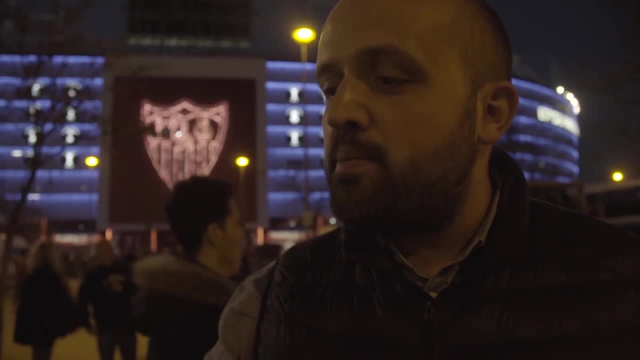 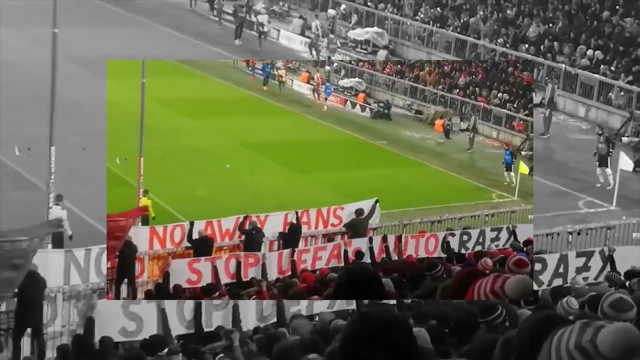 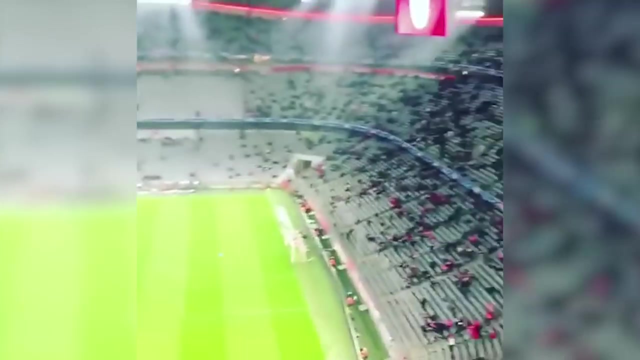 There is not only fight in between us and we can solve it. The problem behind all this is that it's lack of understanding of the fan culture. We just finished things up here in Munich, It's now 6 am and we're flying over to Seville by Lisbon tonight. 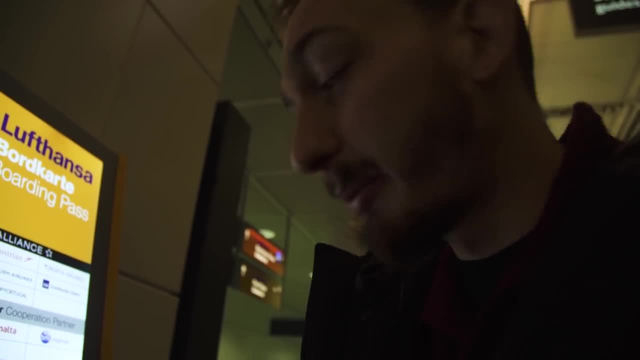 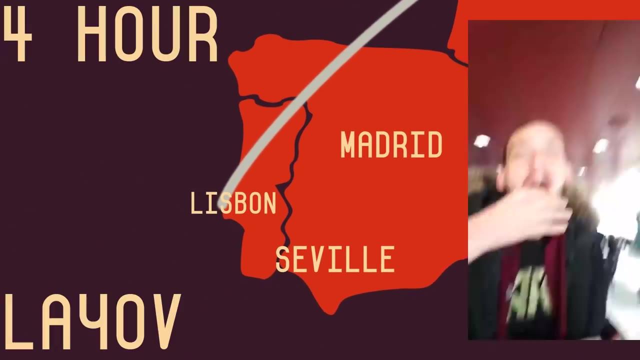 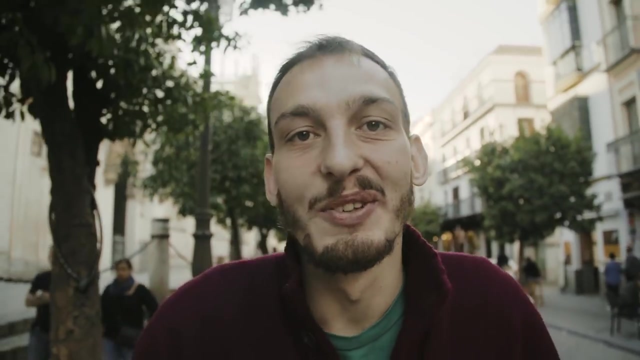 Seville, Manchester United. If you thought this story was ridiculous, get ready for what happens in the next city. Let's go. Ticket prices go up. So now we're in Seville, Spain. We're going to meet up with the Manchester United supporters for starters. 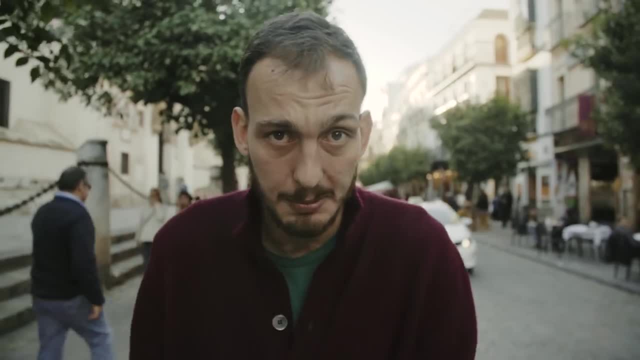 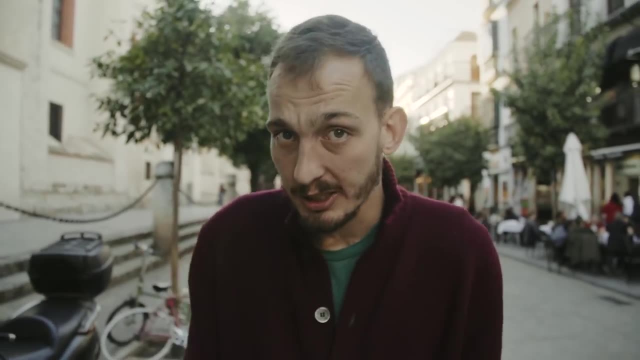 They're going to tell us about how they're working with the club to make sure the tickets are subsidized and they can stop getting screwed over when they're travelling abroad for UEFA matches. All of them are calling on one thing, which is UEFA to finally make some legislation to make sure that clubs can't keep screwing over fans when it comes to international matches in the most exciting tournament in the world. 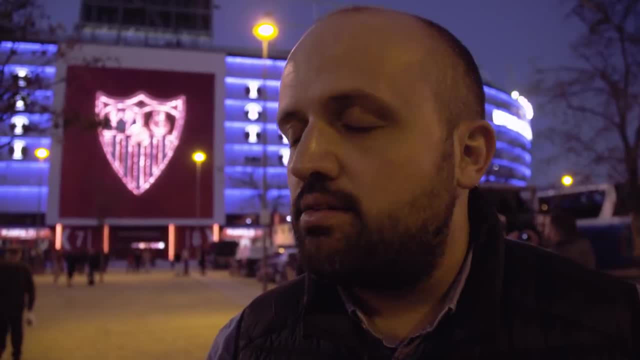 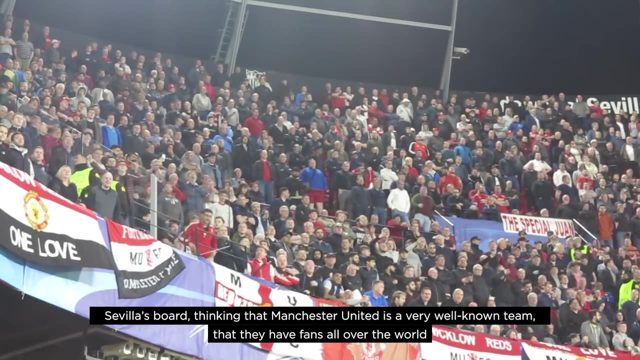 Seville started by deciding to charge United fans 100 euros for this match. The management of Seville, thinking that Manchester was a well-known team, that they had fans all over the world, raised prices disproportionately to 100,, 150, 200 euros. 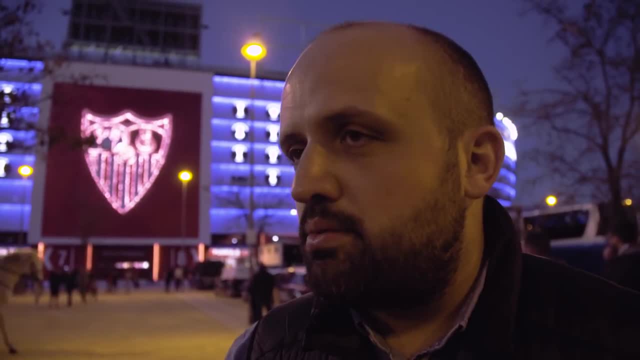 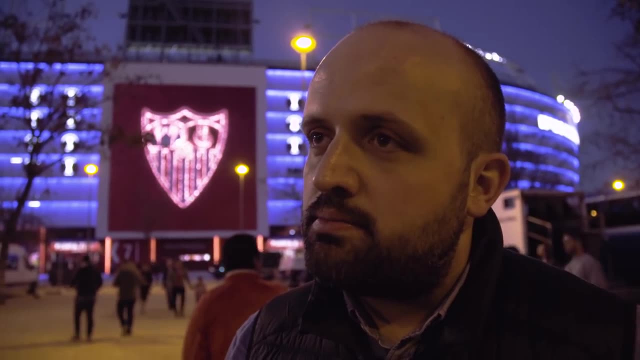 The proposal from United was originally 60 euros, which seems to be a rather reasonable price. So they fought the case with Seville and they said, no, you shouldn't be charging that much. Clubs were not able to reach a reasonable agreement. 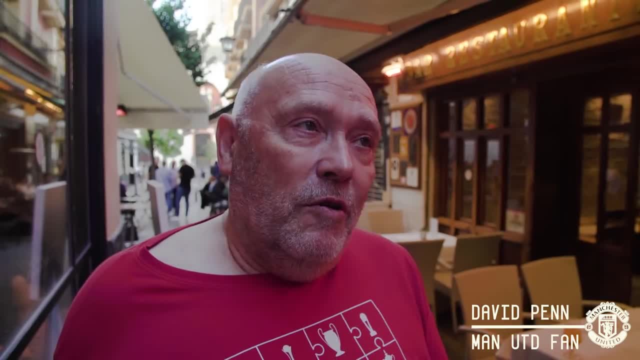 Our club, I know, gave them an ultimatum and said: look, if you don't, what we're going to do is we're going to charge your fans 100 euros, but we're going to give the extra money back to our supporters, so they only pay 100 euros. 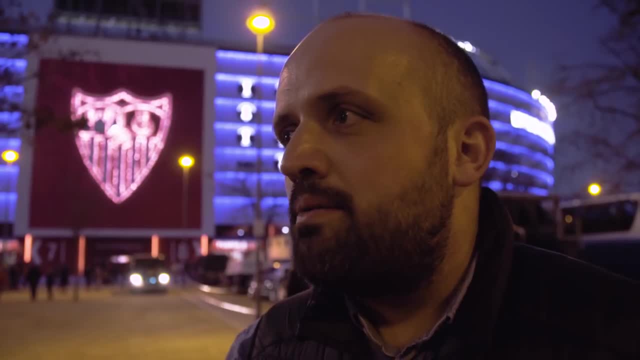 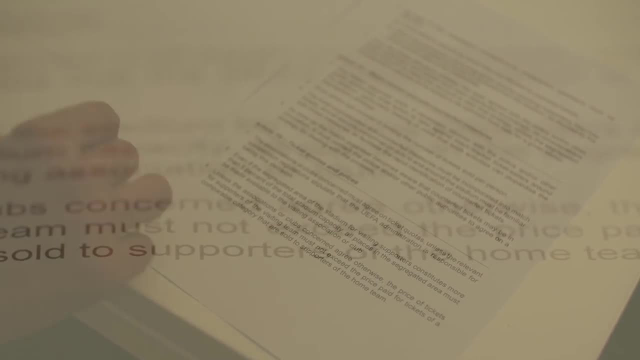 We're not going to pay as much as Liverpool did. It's quite significant how a stronger regulation is needed. Hold them is the way the regulation is written. it allows some clubs to take advantage and say: well, actually, strictly, we're still following the rule. 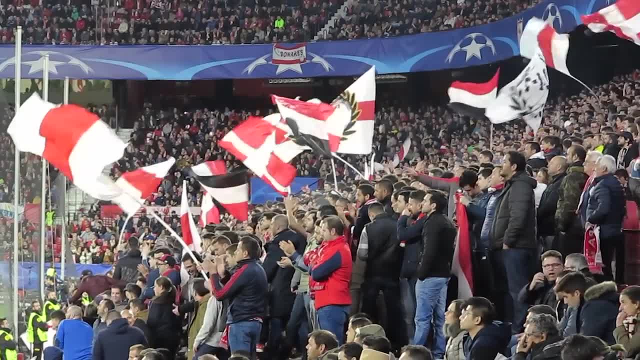 There are so many loopholes around it. You can, for example, give a discount to your members, which is often what a Spanish club do because they have a lot of members. You can sell tickets in a bundle, which is what unelected 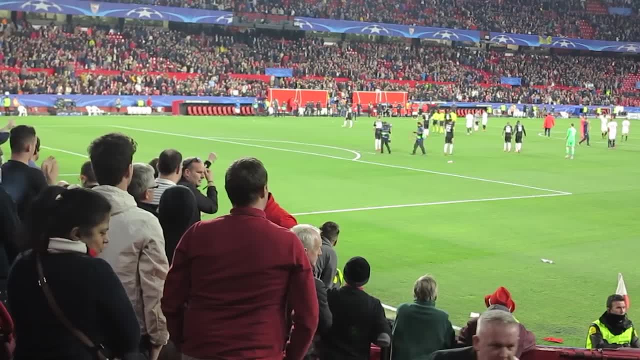 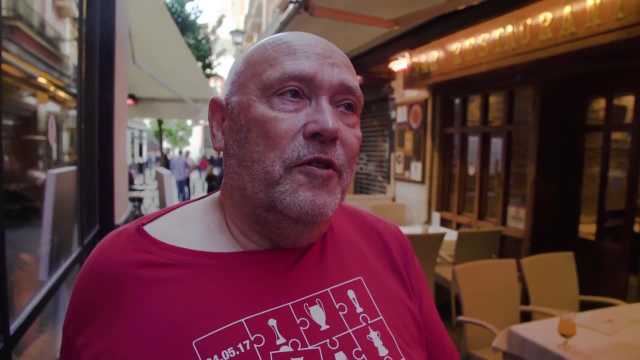 So clearly the regulation is not sufficient. It needs to be amended, It needs to be more specific and it needs to take into consideration that clubs are not always reasonable. Now we're not sure what's going to happen next, because we know there was this successful disciplinary case against Anderlecht. 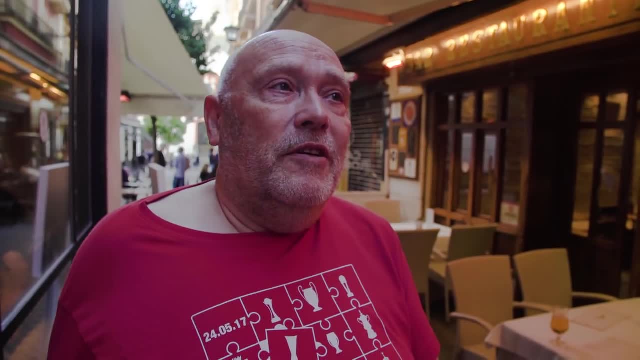 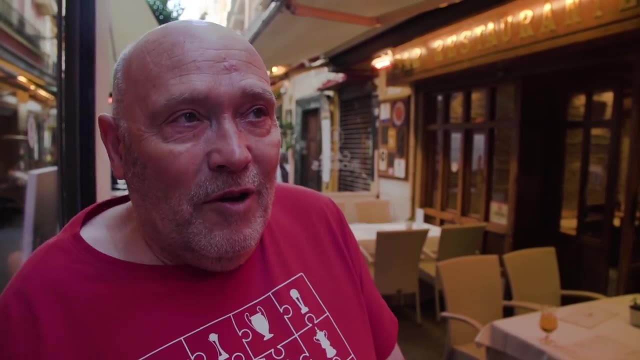 But we want to make sure there is absolutely no doubt. So change the regulation, make it more specific, make it clear that we don't pay any more than season ticket holders or their equivalent in that part of the season. How many pesos? One hundred?